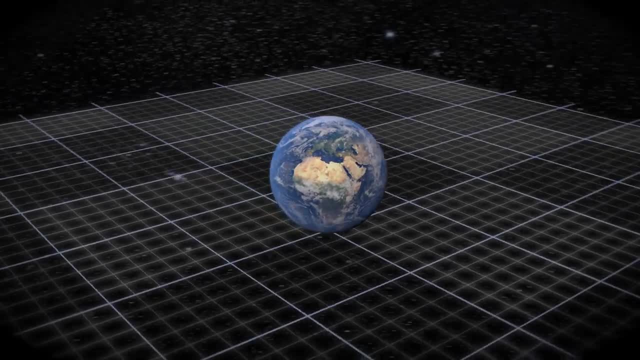 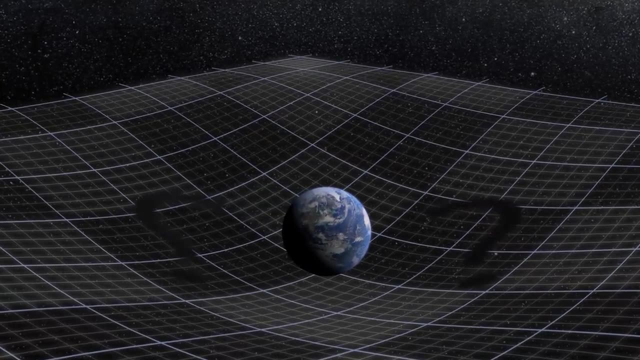 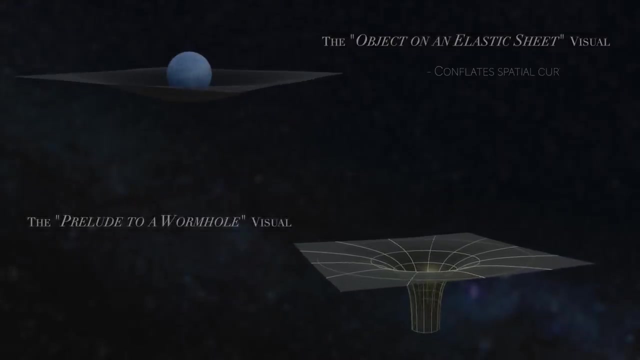 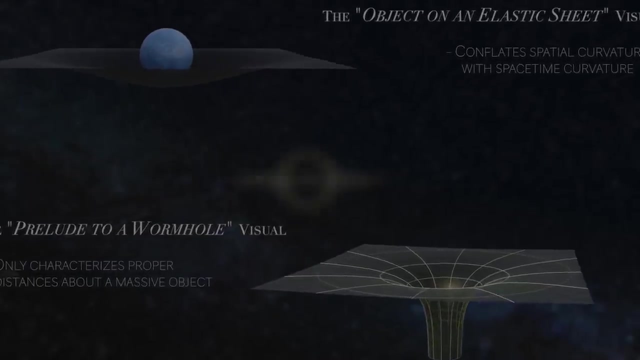 We're often told in physics that the presence of massive bodies warps the fabric of space and time, But what does such a statement actually mean? Most visuals are heuristic tools that don't offer clear understanding, Leaving one to wonder: is it possible to actually visualize space-time curvature? 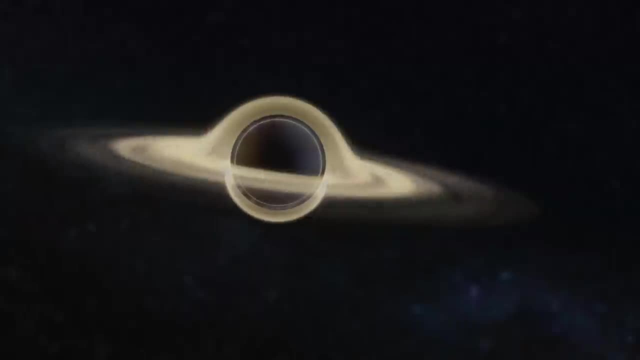 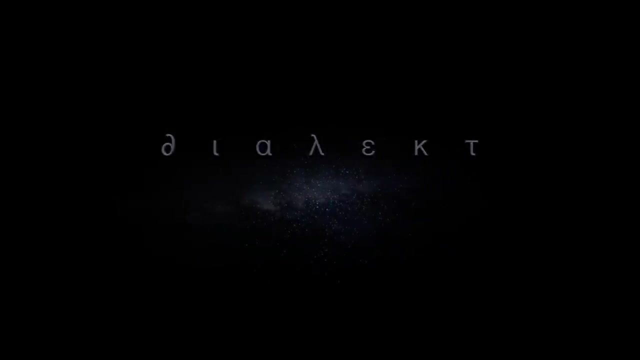 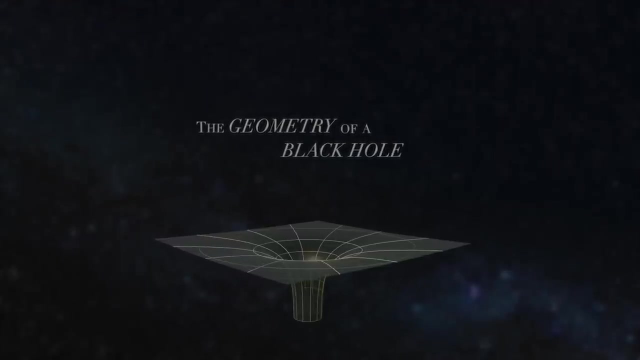 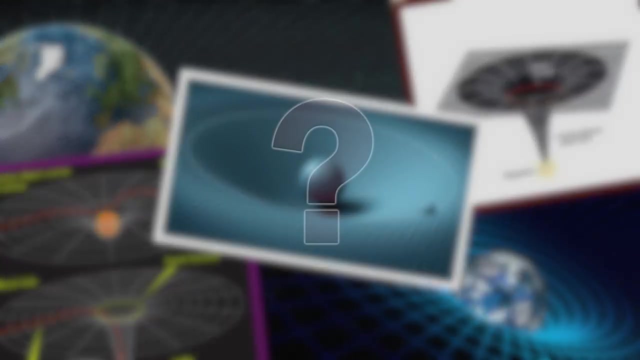 especially near an object so massive we can cross a limit of no return. This is DIALECT with The Geometry of a Black Hole. What does the curvature of space and time around a massive body actually look like? To answer this question, we need to turn to a mathematical object called the Schwarzschild metric. 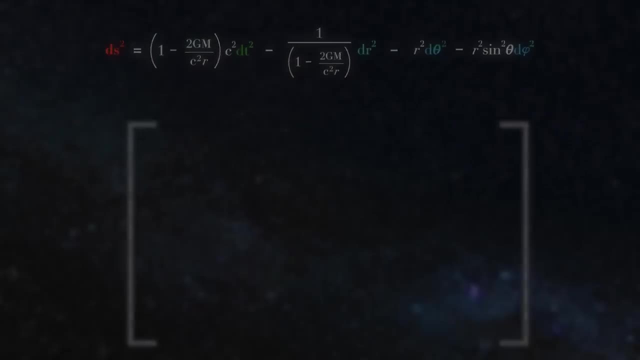 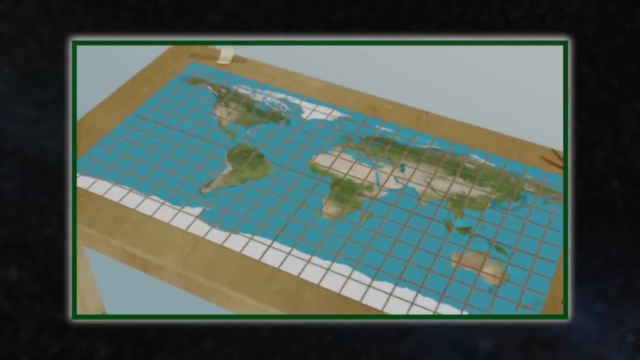 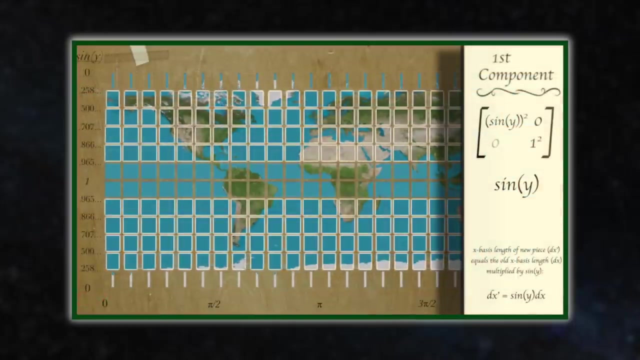 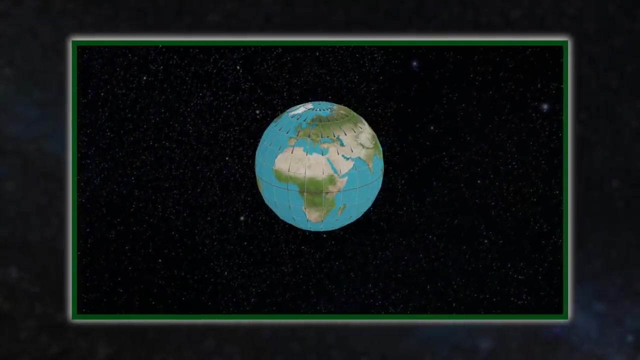 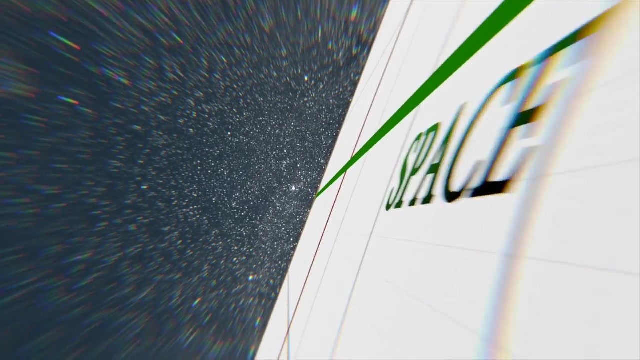 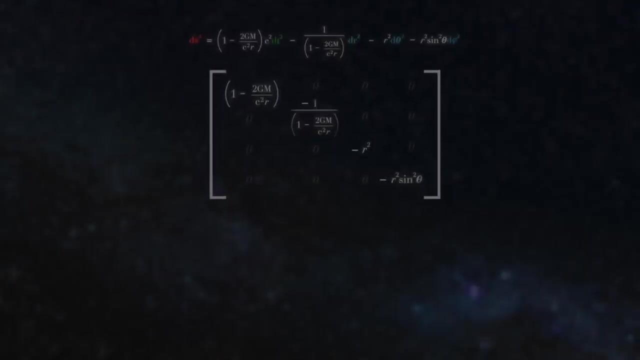 Presented in tensor form. this metric is a matrix with four expressions along its diagonal components. Now, in our prior videos, we demonstrated how the components of a metric tensor can be interpreted as instructions for writing. This is a basic method of re-sizing infinitesimal pieces of a map in order to fit those pieces to a curved surface. And indeed this is the case whether your map is one of a physical surface like that of the earth, or whether it's a map of a more abstract surface like that of the space-time manifold. We can thus use the Schwarzschild metric to construct for ourselves a model of curved space-time. 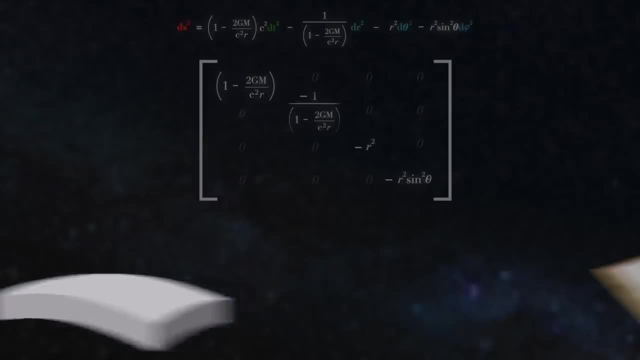 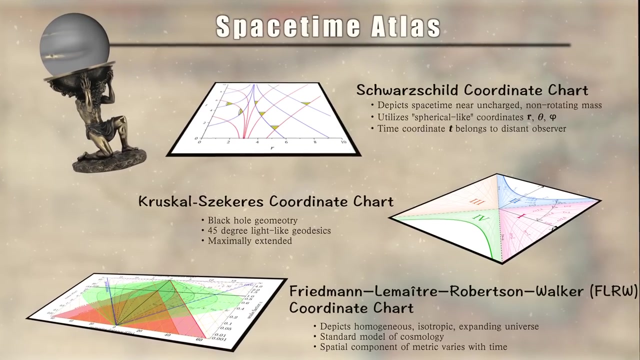 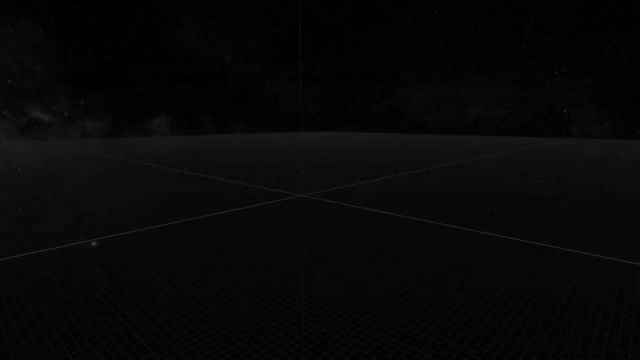 But first we must get our hands on the map which the metric belongs to. Here we turn to what's formerly known as the Schwarzschild coordinate chart. This map depicts spacetime in the vicinity of a single, centrally located, non-rotating 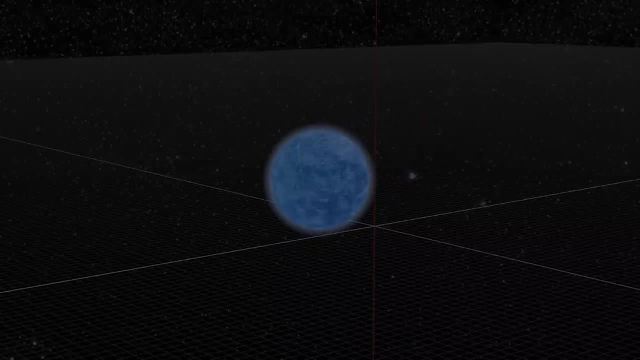 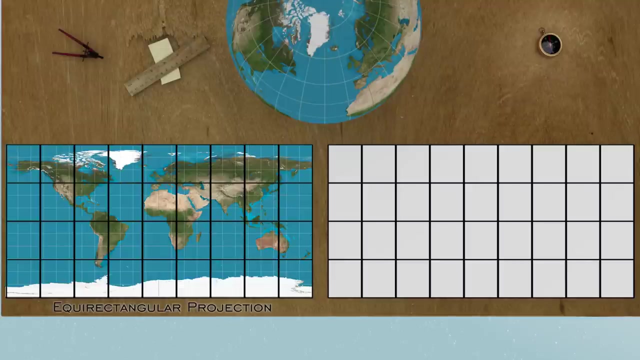 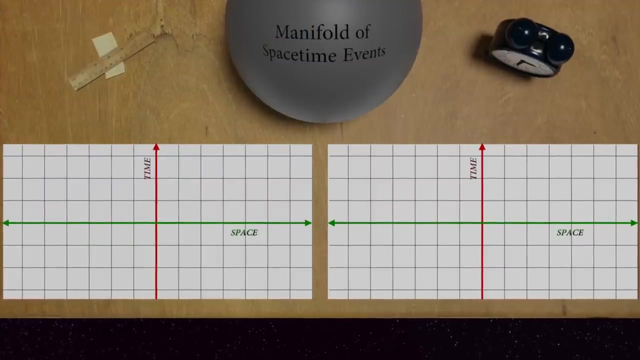 uncharged spherical mass. Now, just as there's no one right way to map out the curved surface of the Earth onto a two-dimensional Cartesian grid, there's no one right way to map out the curved surface of spacetime onto a four-dimensional Cartesian grid. 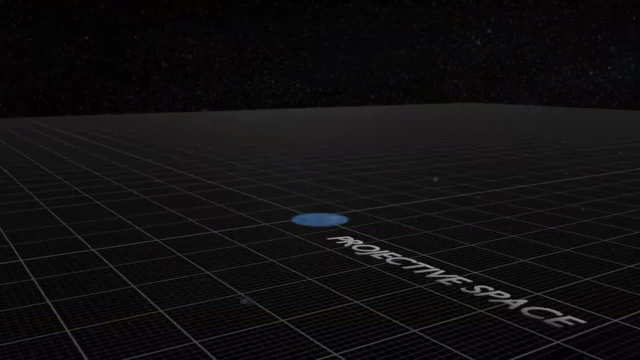 Consequently, we have a choice in how to make such a projection, Motivated by the spherical symmetry of the region. the Schwarzschild coordinate chart is a perfect example of how to map out the curved surface of the Earth onto a two-dimensional Cartesian grid. 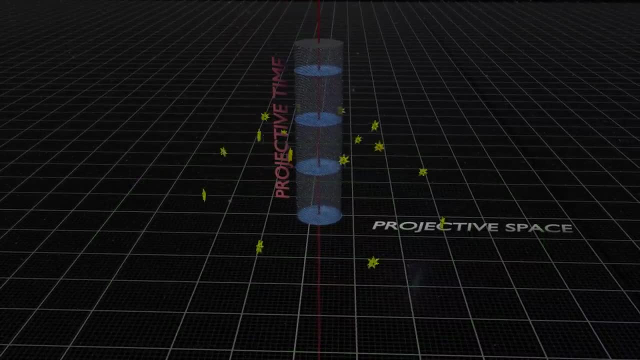 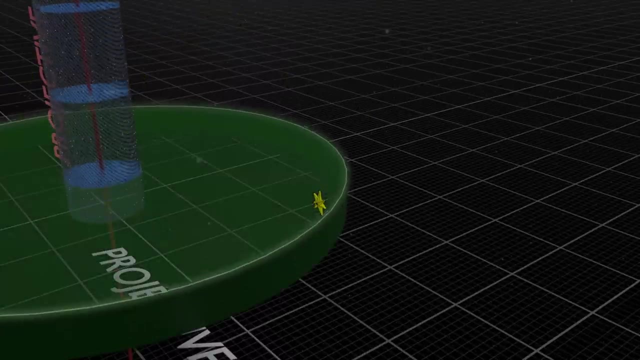 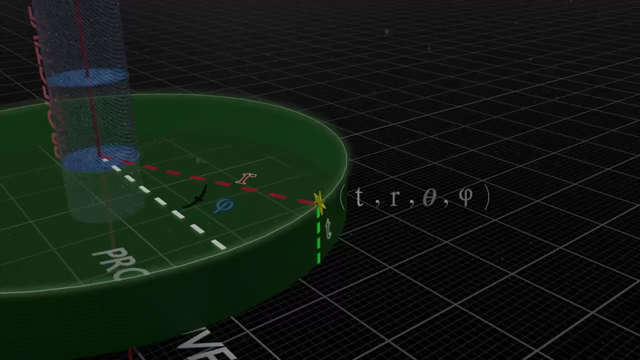 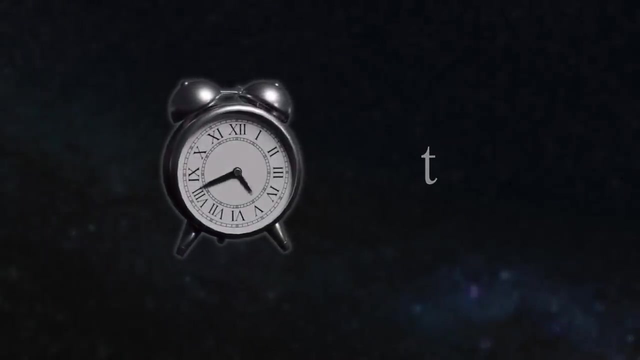 Consequently, we have a choice in how to make such a projection. The Schwarzschild approach is to assign to every world event that occurs a set of more or less spherical-like coordinates. The first coordinate, t, is intended to be analogous to a traditional time coordinate. 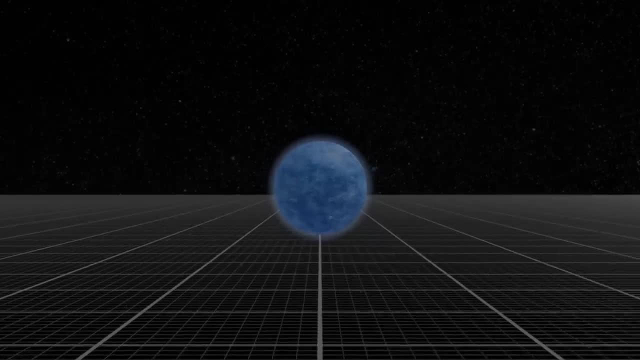 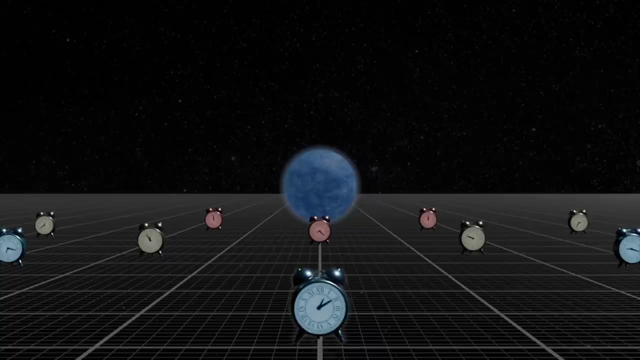 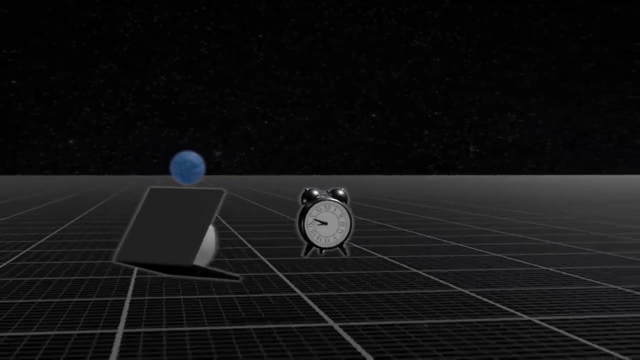 As there is no global time in this region and clocks everywhere tick at different rates, the simplest solution for describing time here is simply to choose a master clock, meaning a clock against which all others can be compared. The natural choice will be that of a clock belonging to a distant observer, since far 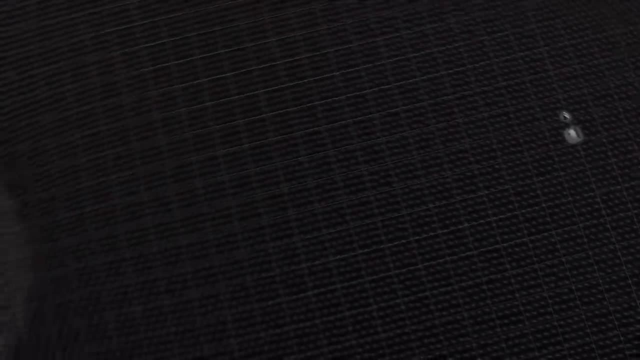 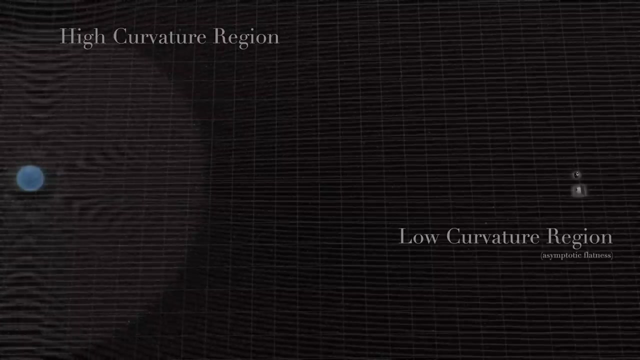 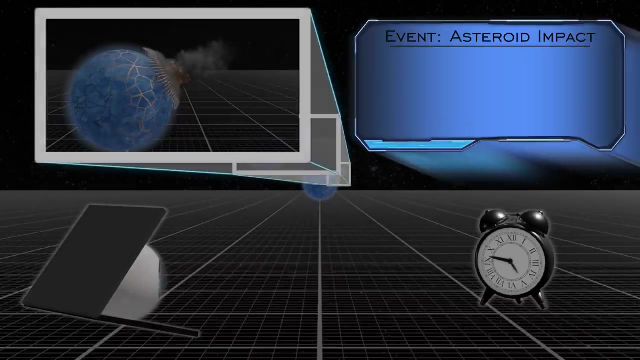 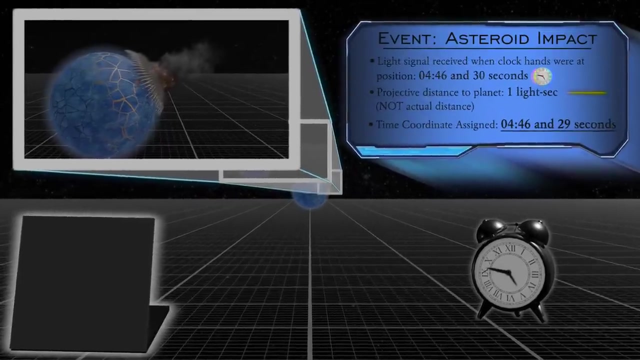 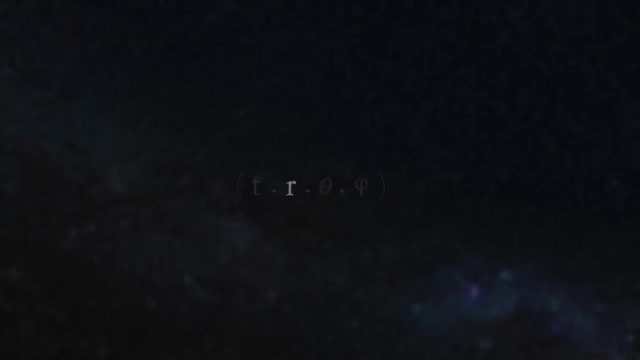 out from the central mass spacetime curvature will be negligible. All events which transpire across this spacetime region are thus assigned a time coordinate based on whenever this distant observer perceives them to occur. The second coordinate, r, is analogous to a radial coordinate. 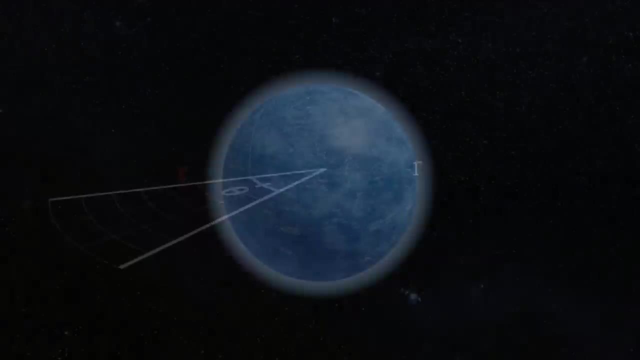 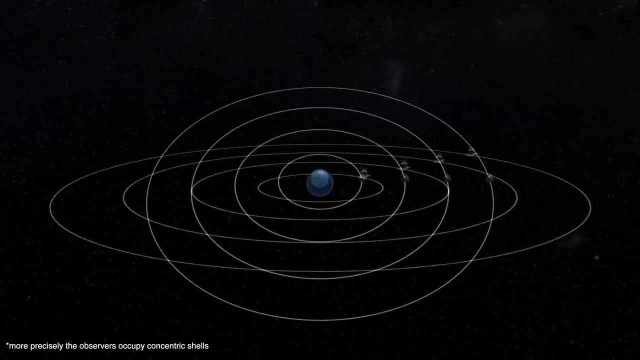 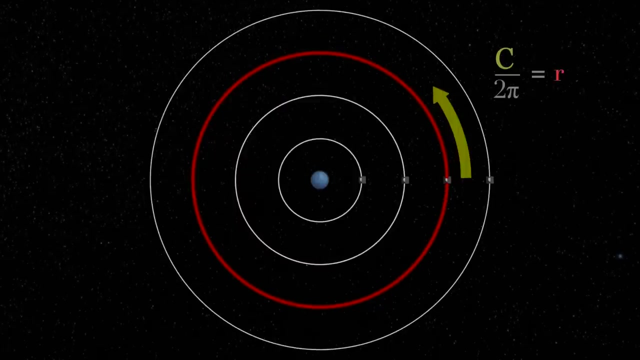 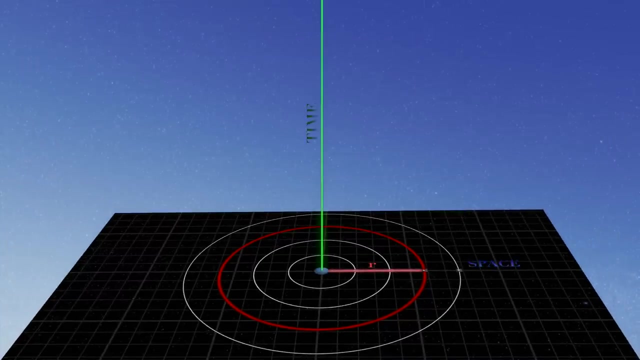 It is produced by placing observers in concentric rings about the mass, then having those observers measure the circumferences of the rings in order to deduce, via dividing by 2 pi, what the respective radii of the rings would be were the overall geometry of the spacetime region there flat. 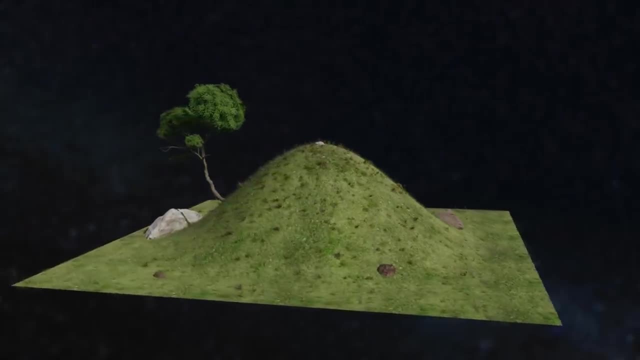 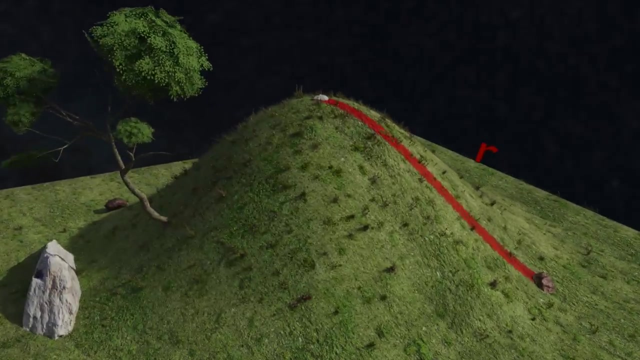 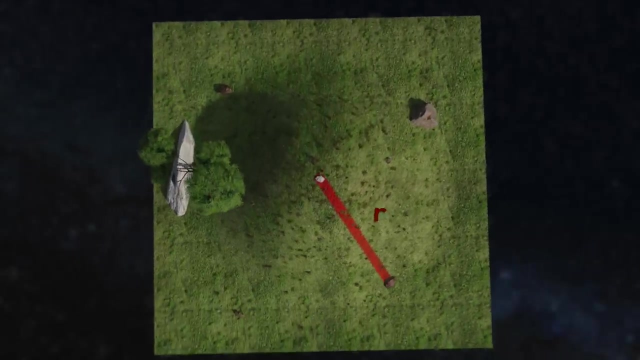 This is like making a bird's eye map of a circularly symmetric hill. The radial distance between any point and the top of the hill obviously depends on the hill's curvature and grade, But once projected onto a flat surface, this distance instead becomes the circumference. 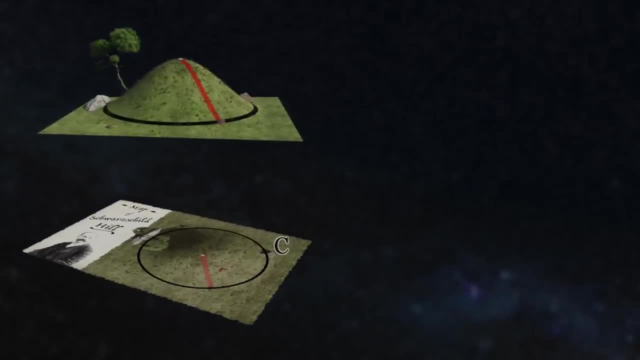 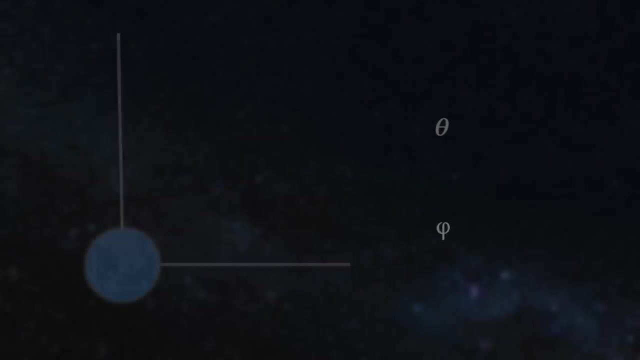 of the contour which the point occupies, divided by 2 pi. Meanwhile, the third and fourth coordinates, theta and phi, retain their ordinary meaning from spherical coordinates as the polar and azimuthal angles about the central mass. Together, these four coordinates, once assigned to every event, map out what time and space. 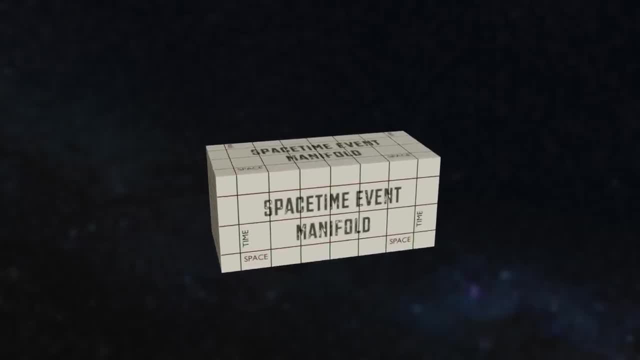 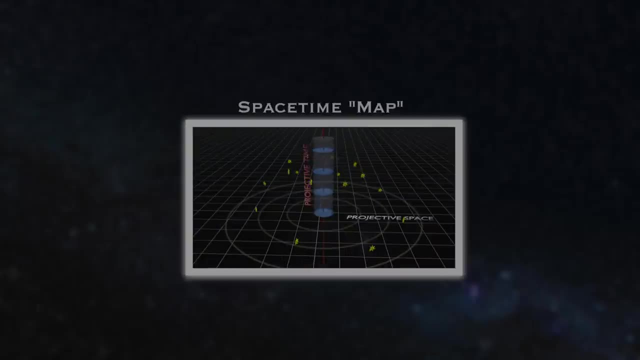 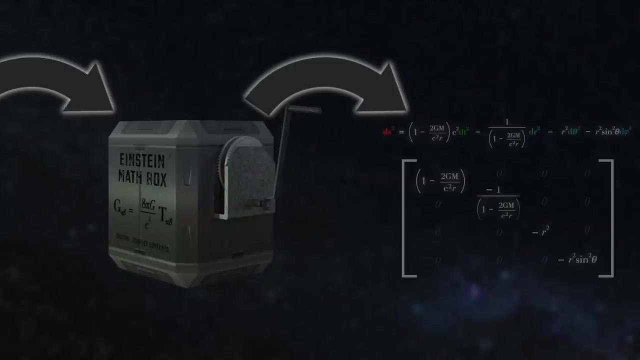 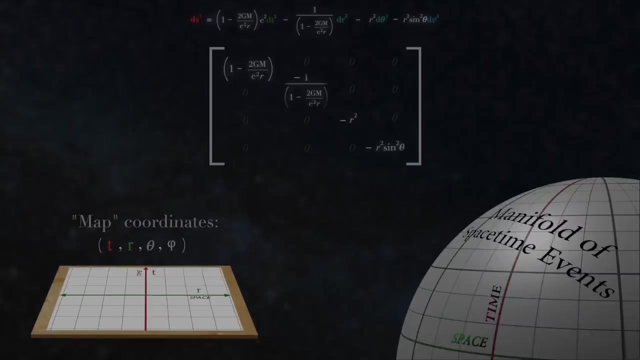 would look like in this region if spacetime were flat. But of course spacetime isn't flat here, It's curved, Which is why, once we feed our map into Einstein's equations, out pops the Schwarzschild metric Telling us how our artificially constructed coordinates relate to the true spacetime geometry. 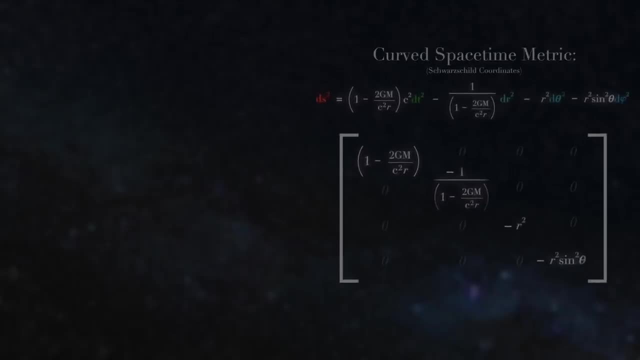 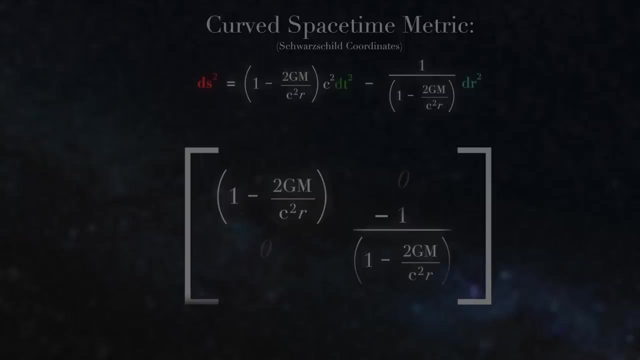 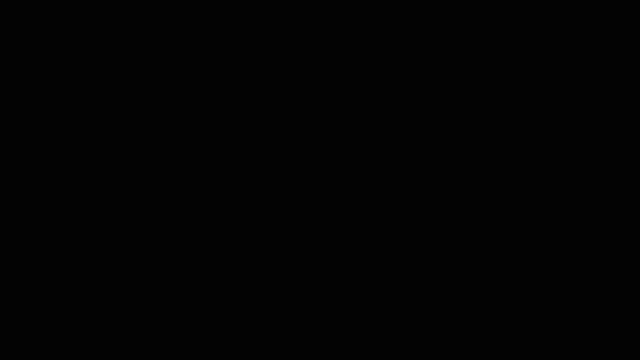 Now, since the last two components of this metric are the same as they would be in flat spacetime time. For the time being, it'll be simpler to drop them from the picture and only consider a two-dimensional spacetime manifold. Don't worry, though, we'll add those dimensions back in later. 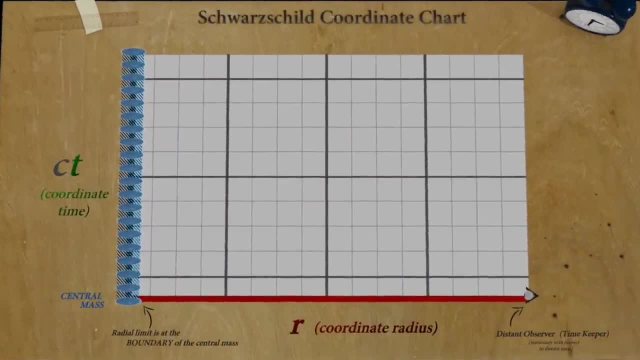 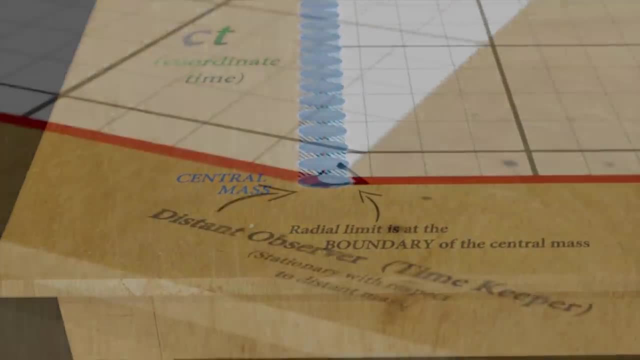 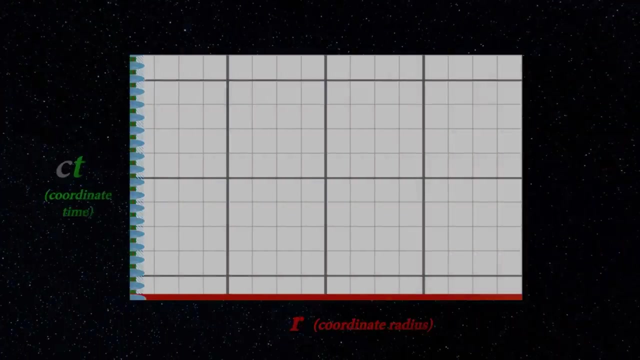 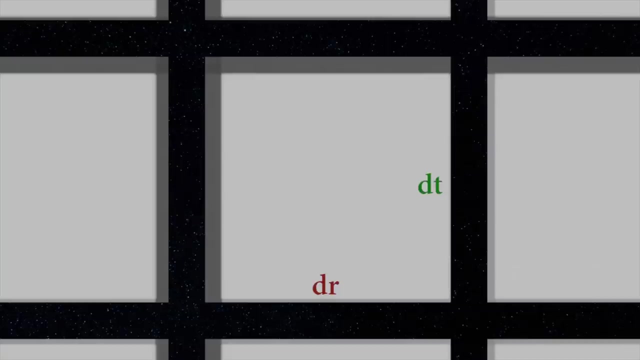 We are now ready to transform our map, ie the Schwarzschild coordinate chart, into an actual spacetime surface. The procedure is simple. To start, we cut the map into many tiny square pieces, dr by dt. Then we simply follow the instructions from the metric tensor. 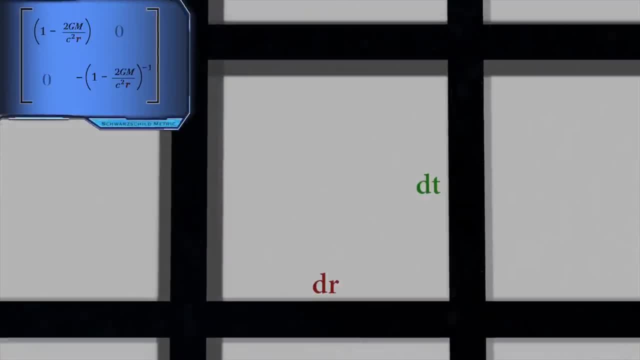 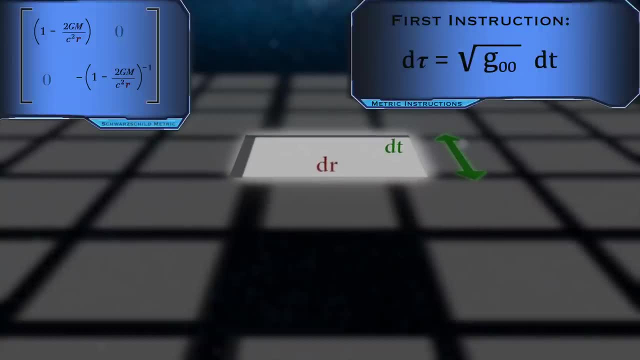 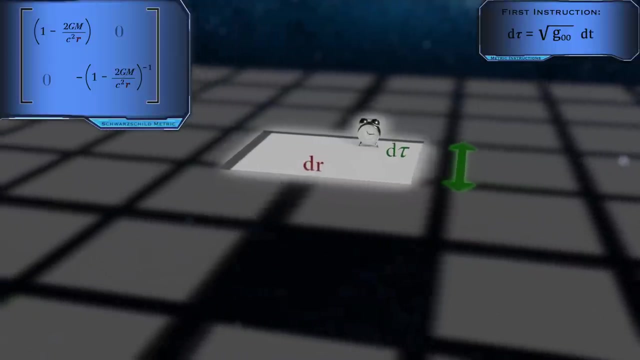 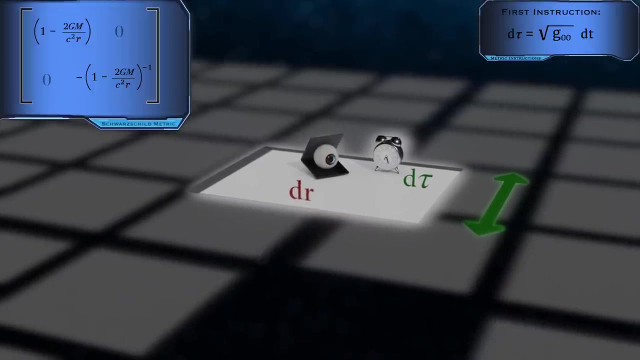 Now the first instruction tells us by how much we need to stretch or shrink The coordinative dt length of each mapped piece in order to match it to its true surface length, ie that length of proper time an observer located there would experience. 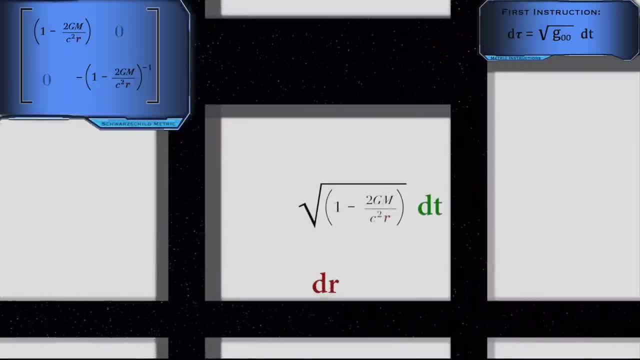 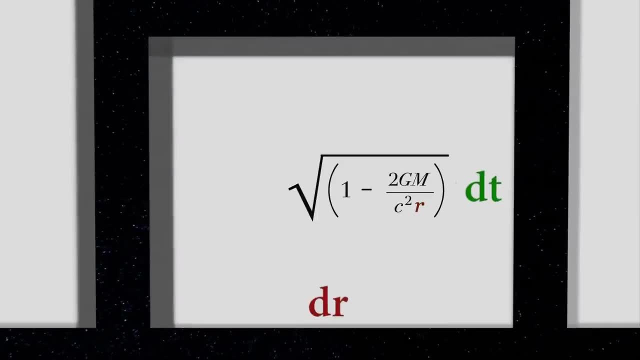 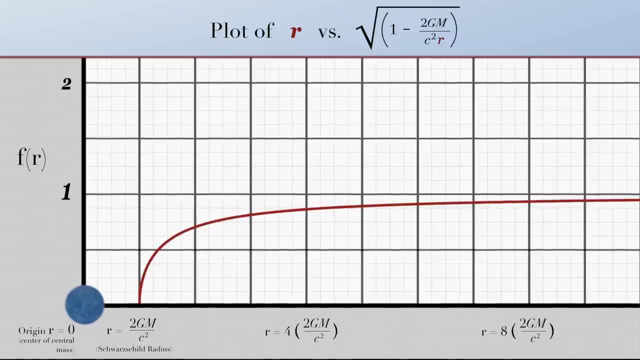 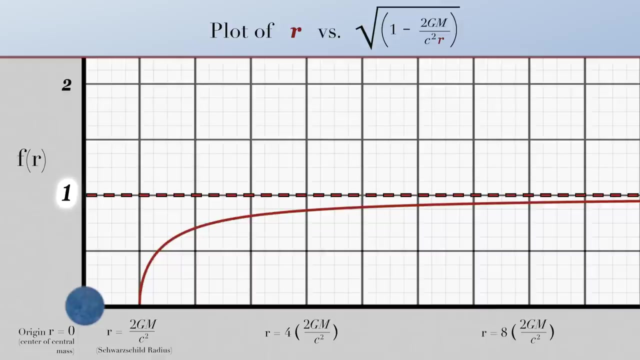 Here that value corresponds to the square root of, divided by c squared times the r coordinate of that piece. We can see that for very large r coordinates this expression takes on a value of nearly 1, meaning that the temporal lengths of pieces far from the central mass will remain essentially. 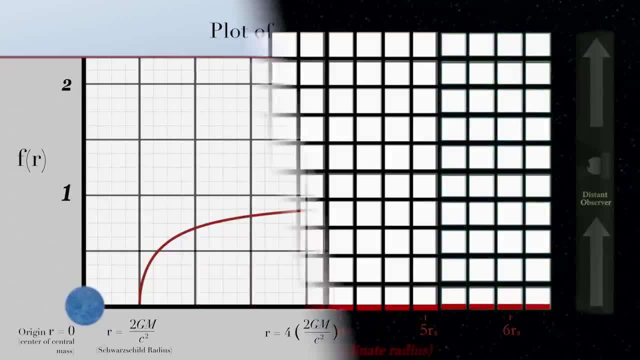 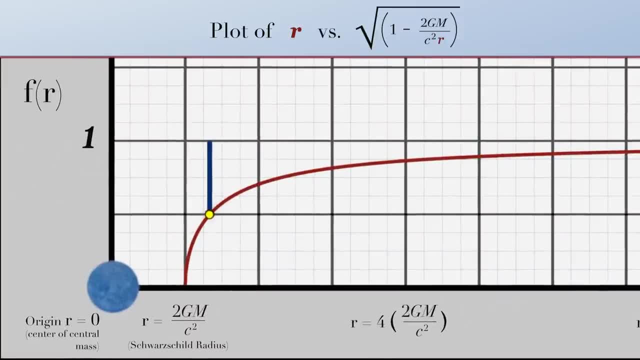 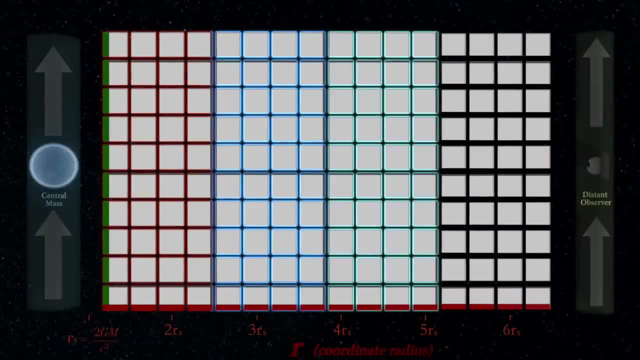 unchanged. For smaller r coordinates, however, this expression takes on values increasingly less and less than 1.. For larger r coordinates, this expression takes on values increasingly less and less than 1. Meaning that the temporal lengths of pieces closer and closer to the central mass will. 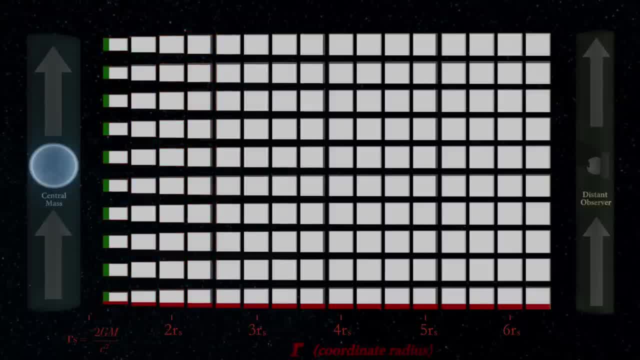 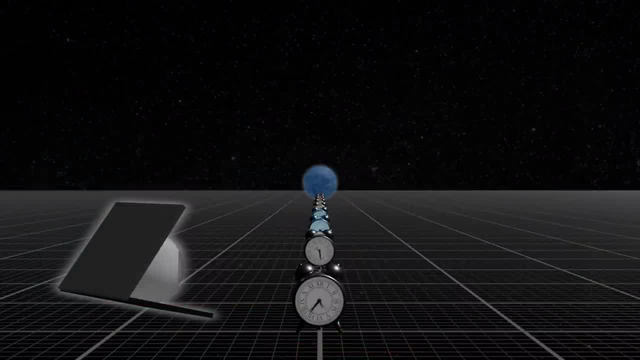 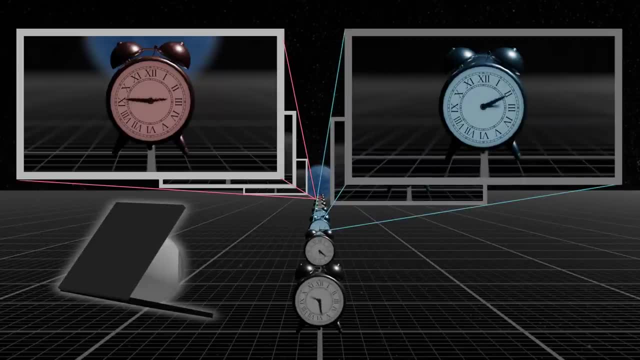 be more and more shrunk. Physically, this means that from the perspective of the distant observer, clocks closer to the central mass will appear to run more slowly than clocks farther away. We can now run with the clock Next 2.. 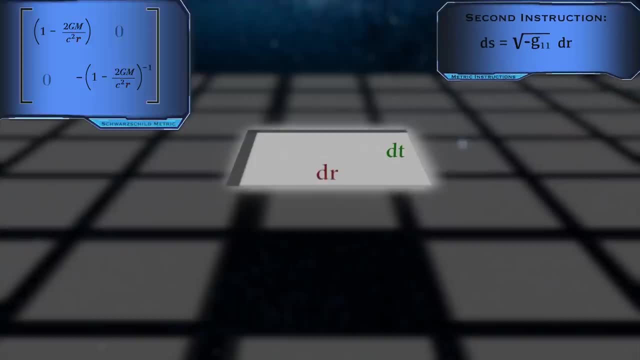 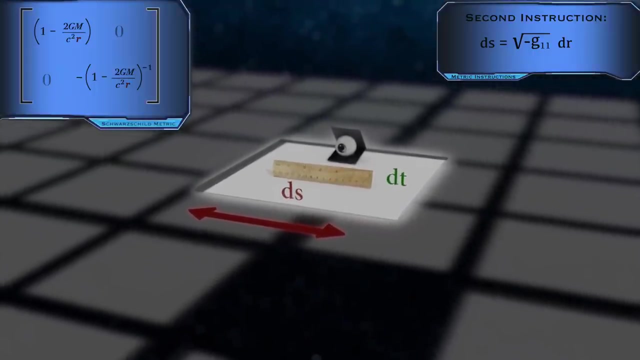 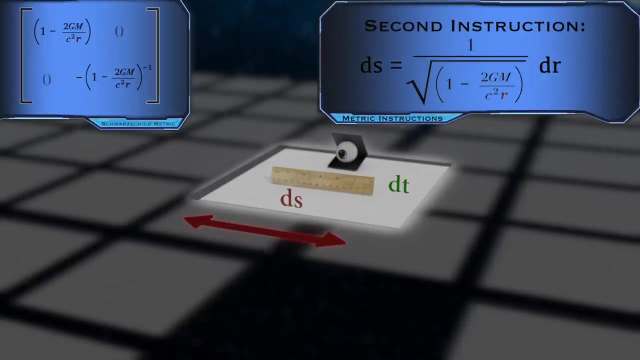 from the metric tensor tells us by how much we need to stretch or shrink the dr length of our piece in order to match it to its true surface length, ie the length of proper distance an observer located there would measure. here that value is just the reciprocal of the former expression, meaning anywhere we saw. 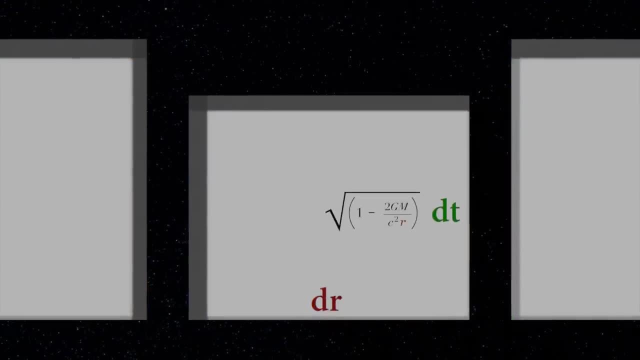 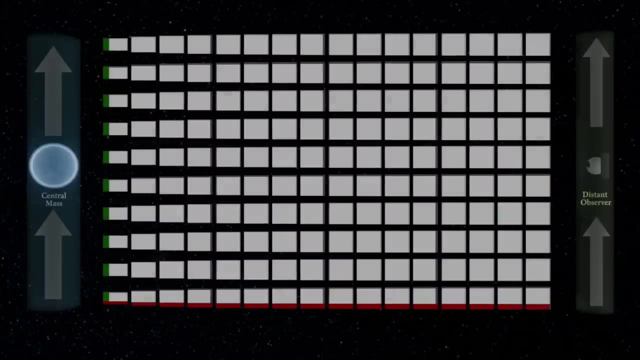 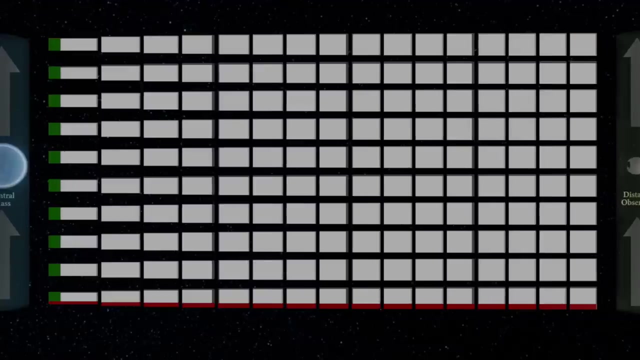 temporal lengths decrease, spatial lengths will increase by the same factor. pieces far from the central mass, then, will, just as with the temporal case, see their spatial lengths remain relatively unchanged, while closer to the mass pieces will see their spatial lengths increasingly stretched. physically, this means that, from the perspective of the temporal case, the spatial length will 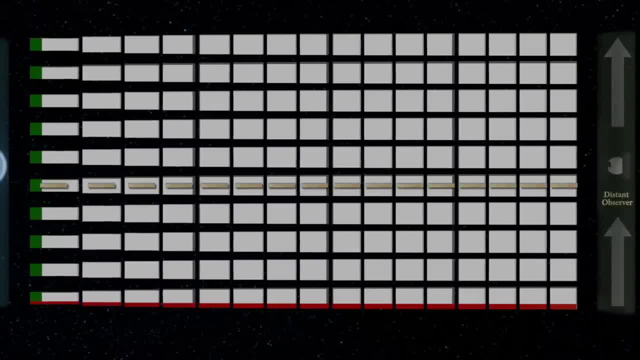 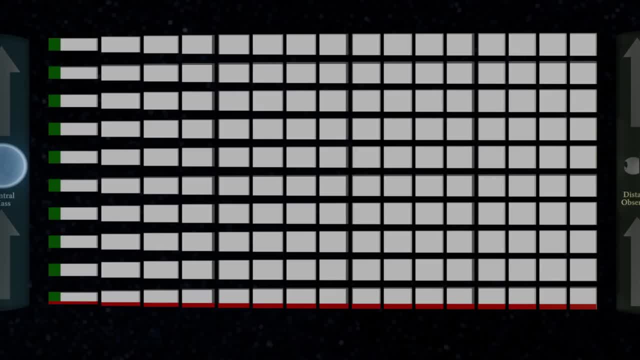 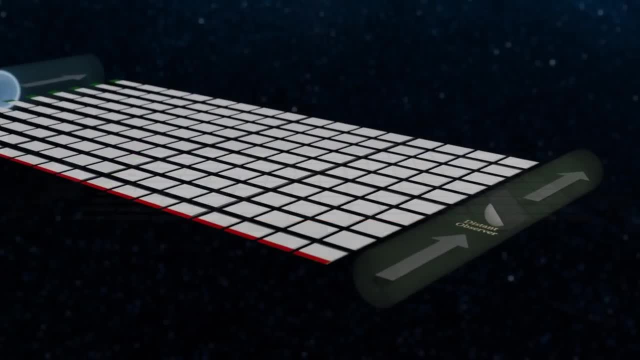 increase with respect to the central mass, between the central mass and the observer and the space time, and here we can see that in this example of a distant observer, rulers closer to the central mass will appear more and more contracted. we now have all the correctly resized pieces of our space-time map. 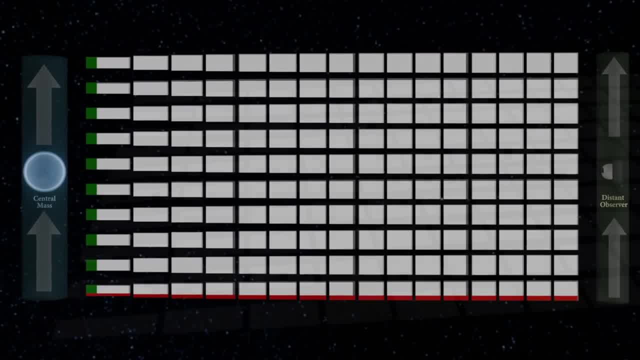 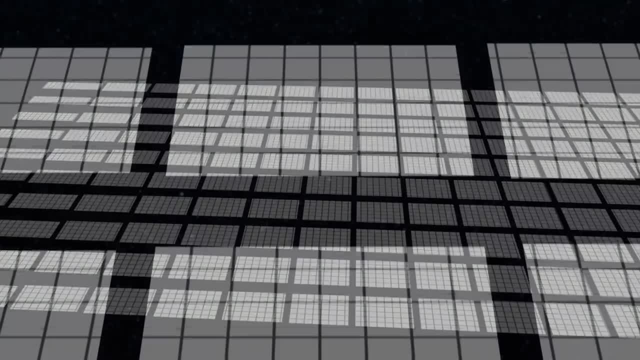 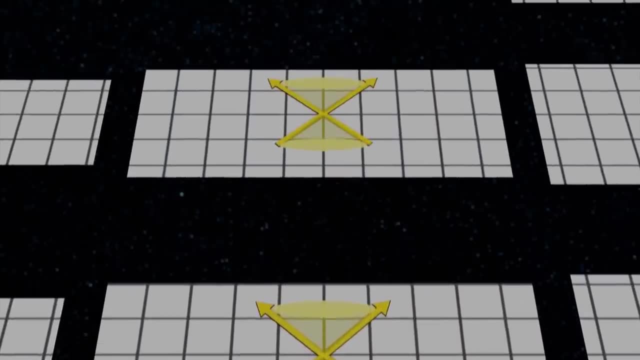 meaning we are looking at our spatio-temporal reality in its true proportions. at this point, let's draw in proper space and time grids on each piece. This will help us understand how the flow of time and space will look across different points of the manifold. Now, although we lack a 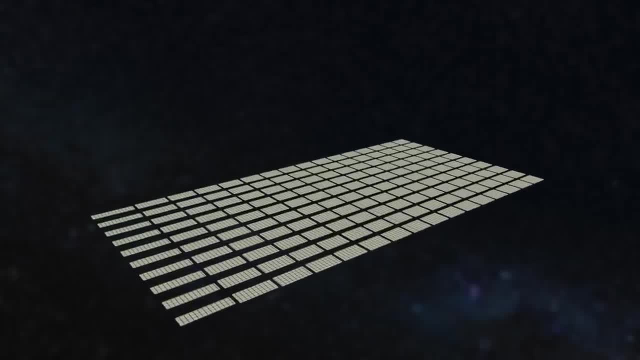 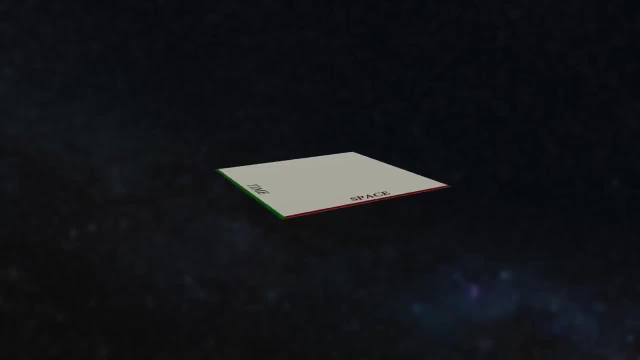 meaningful higher dimensional coordinate transformation with which to appropriately reassemble these pieces. thanks to the fact that we have suppressed the other two dimensions of space, we still have a third dimension left over to play with. Although we can't interpret this extra dimension as anything real, there's no reason we can't use it to aid in our visualization. 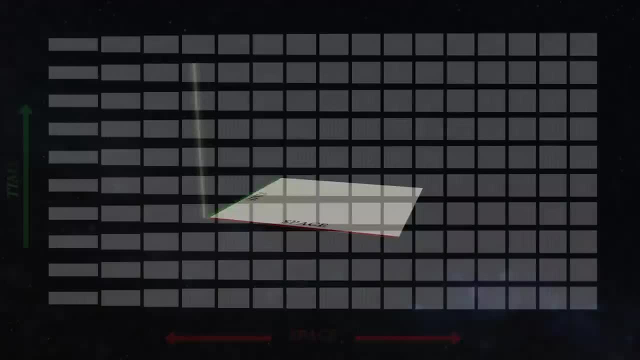 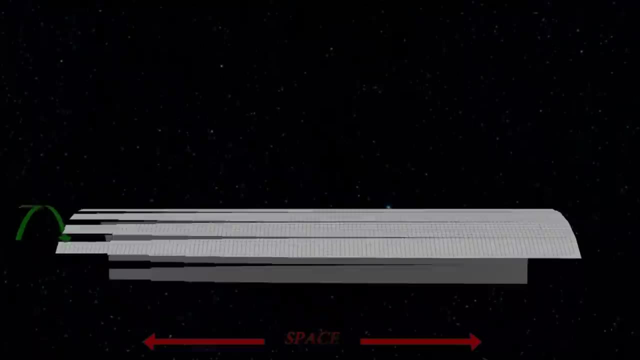 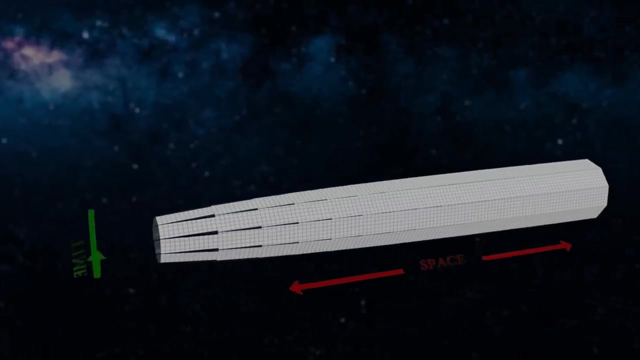 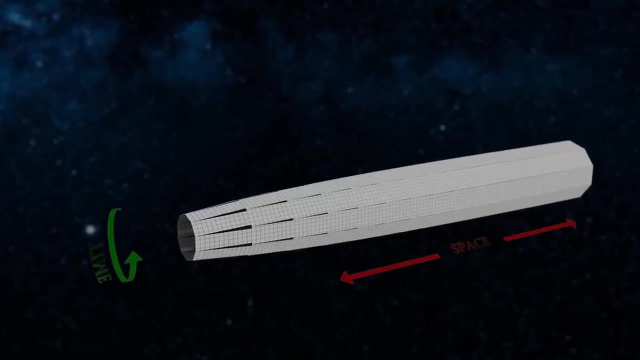 either. So let's put the puzzle together. The trick here is to first roll the entire surface up in a cylindrical fashion and then to bend the tapered edges in towards one another until adjacent pieces are formed. And voila, there we have it. What the curvature of spacetime in the vicinity of a 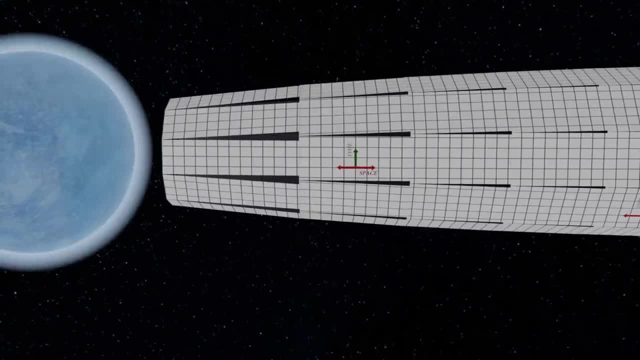 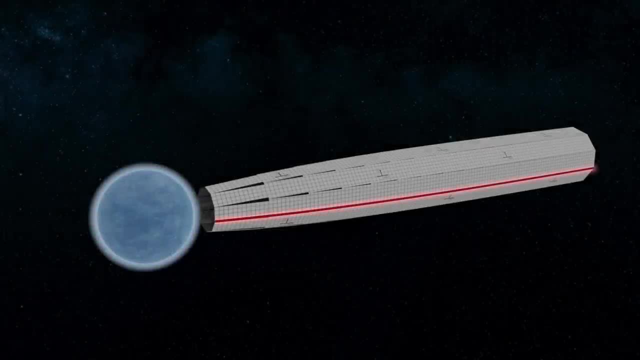 massive object actually looks like. Now note here that where the surface curves around, it doesn't actually rejoin itself. Rather, as we move along the temporal direction, we can imagine the surface getting continually rolled up like a large sheet of paper. 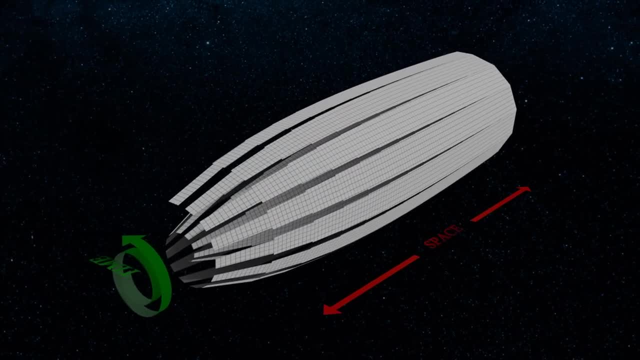 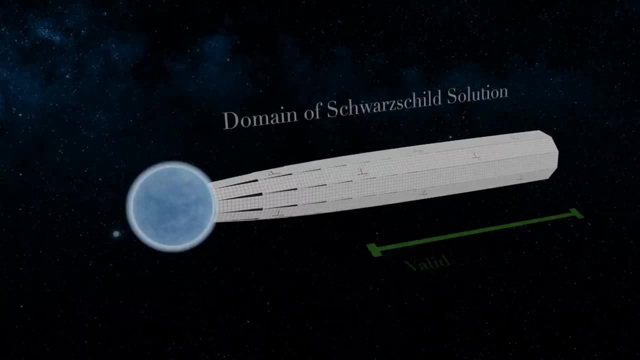 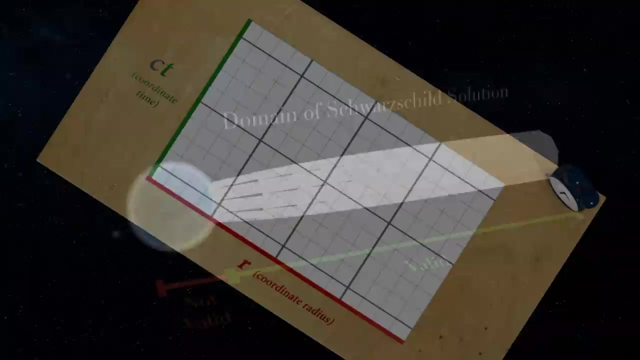 Also note that the boundary of the manifold lies at the edge of the central mass, as the Schwarzschild solution can't be extended to the mass's interior. Lastly, to make this picture more accurate, we can repeat this process with smaller and. 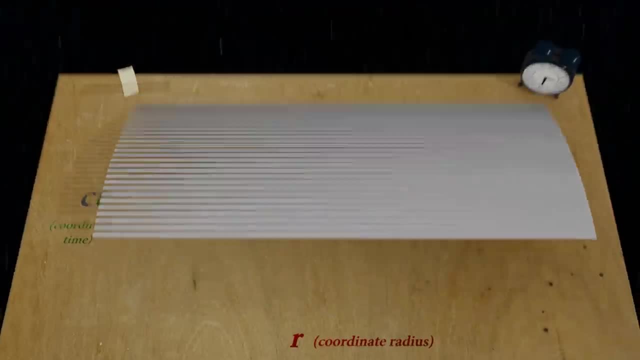 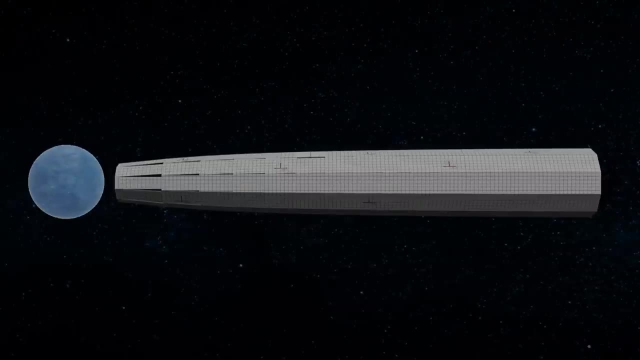 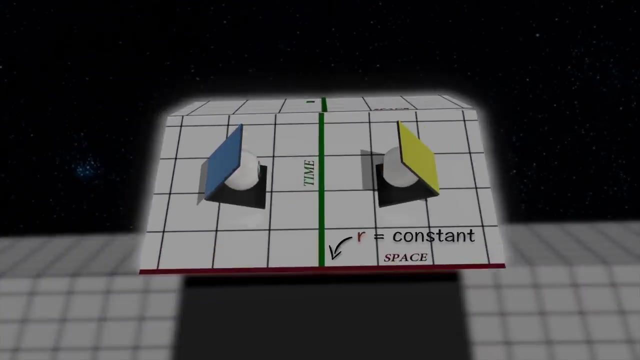 smaller pieces until we essentially have approximated a smooth manifold. So if we want to make this picture more accurate, we can repeat this process with smaller and smaller pieces until we essentially have approximated a smooth manifold. Next, let us consider the motion of two distinct observers sitting together out at some coordinate radius R on this manifold. 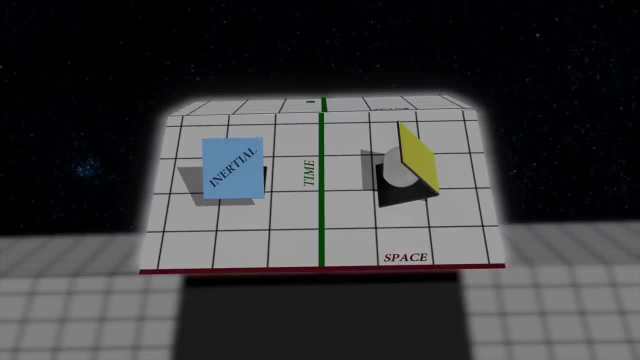 One observer is inertial or free falling and the other is accelerating in order to maintain constant radial distance from the mass. Over a very short period of time, they follow the same world line, together up on the manifold, But in the next instant, the velocity of the accelerated observer. 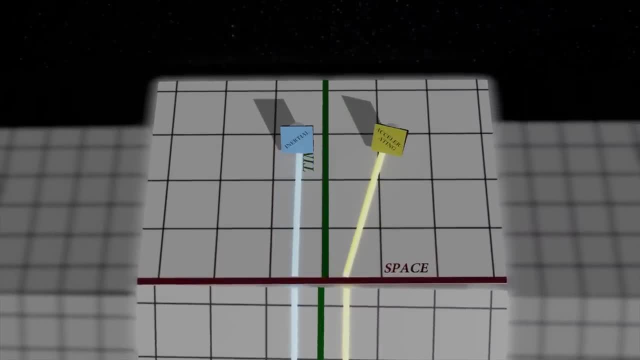 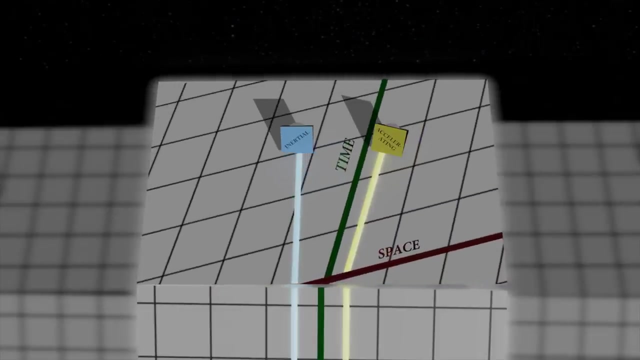 increases with respect to the inertial observer, and their world lines diverge. Now. the proper grid on this next manifold piece depicts space and time as measured at a constant radial distance, meaning it belongs to the accelerated observer, not the inertial observer. Thus we must transform into the frame of the accelerated observer. 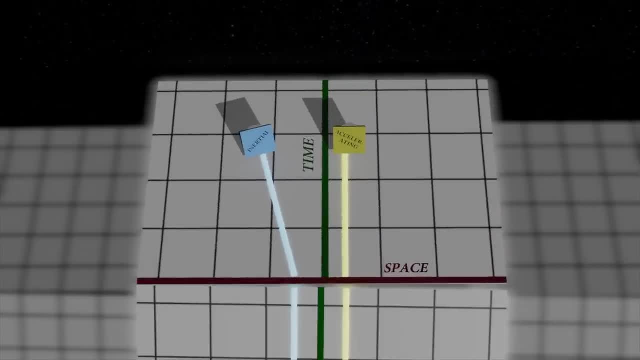 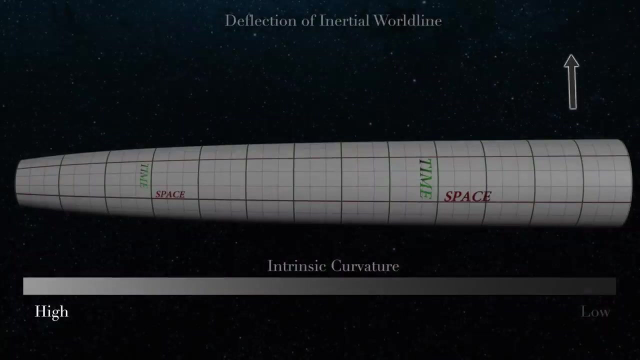 which results in the inertial observer's world line being deflected inwards towards the central mass. High up along the manifold, where the curvature is weak, the amount of this deflection will be very slight, but further down it becomes more and more substantial. 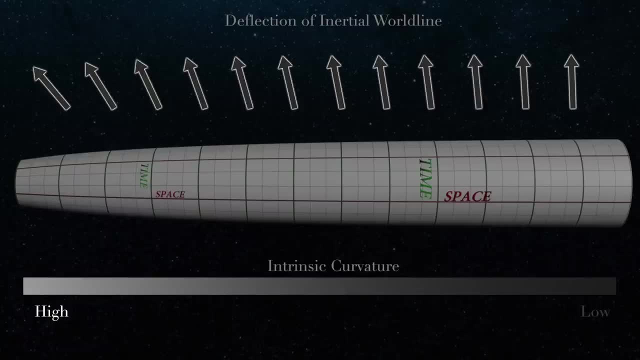 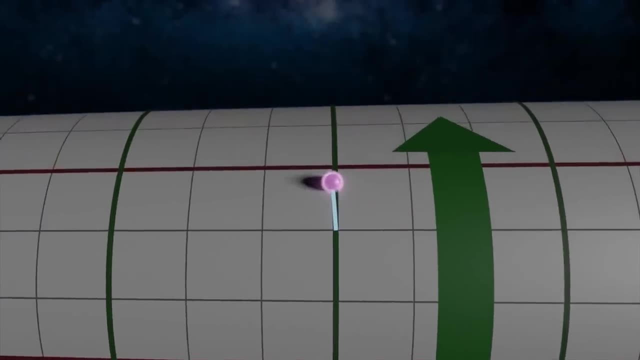 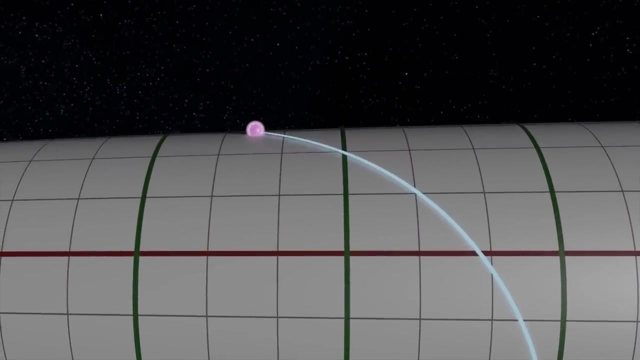 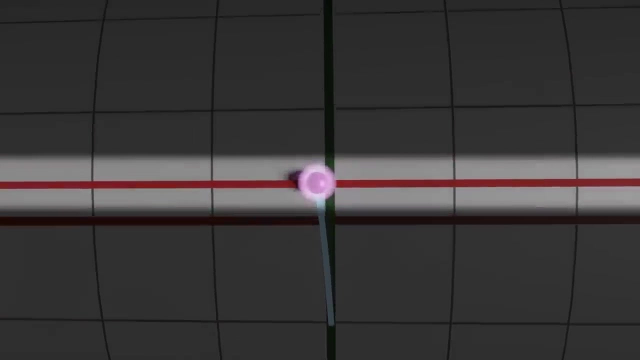 The curvature of the manifold soon helps redirect it down towards the central mass. To see this better, we can keep the object on a constant radial line and depict the progression of time as a rolling of the manifold, as though it were being rotated about an axis running through. 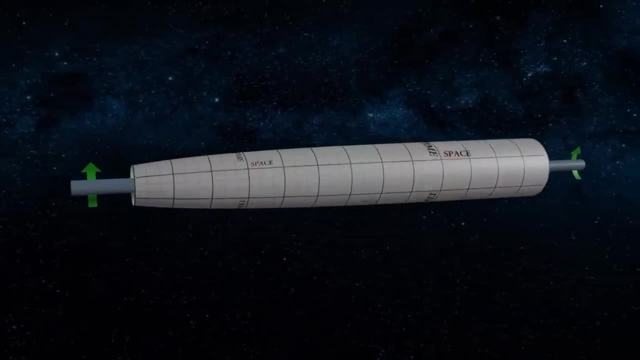 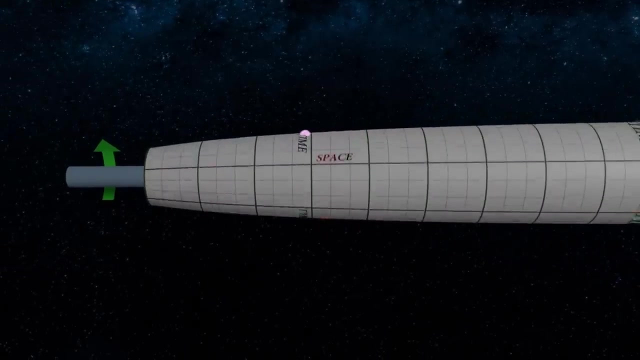 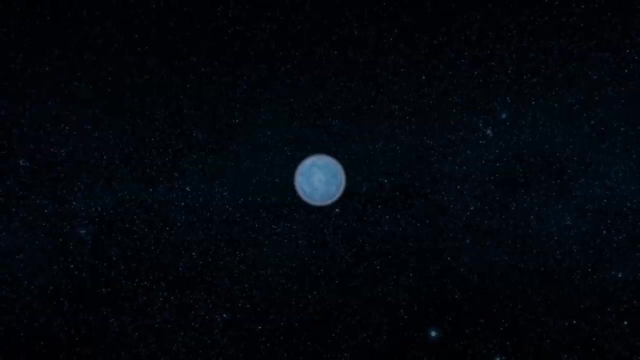 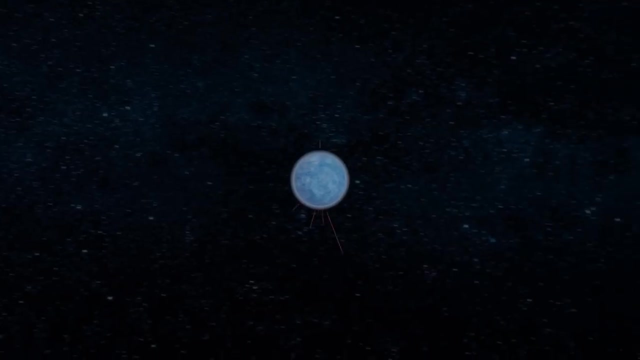 its center. From this perspective, as the manifold rolls forwards in time, the object begins to fall faster and faster down towards the central mass. Next, we can add our missing spatial dimensions back into the picture. To do this, we first draw radial lines outwards from the mass, then we attach a rolling manifold. 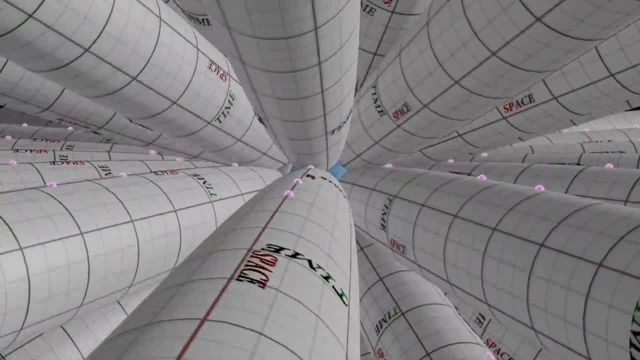 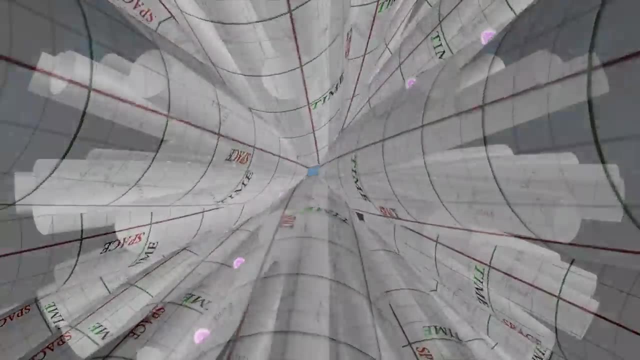 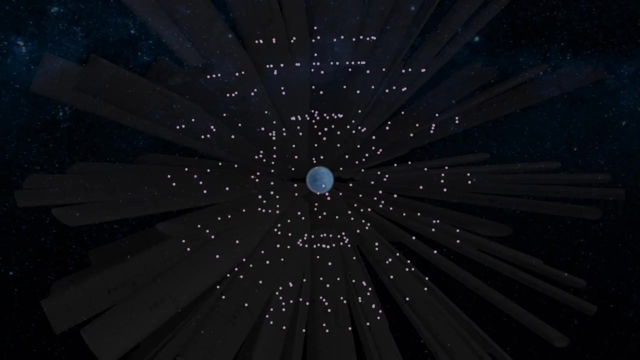 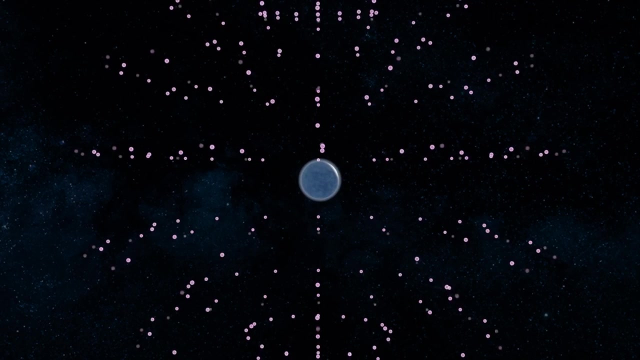 to each line. The visualization gets a bit awkward here, as we are superimposing multiple manifolds atop one another, but next we sort of squash out the temporal rolling, leaving only a visual of the radial motions. We now see that we have a three dimensional space where all objects fall steadily inwards. 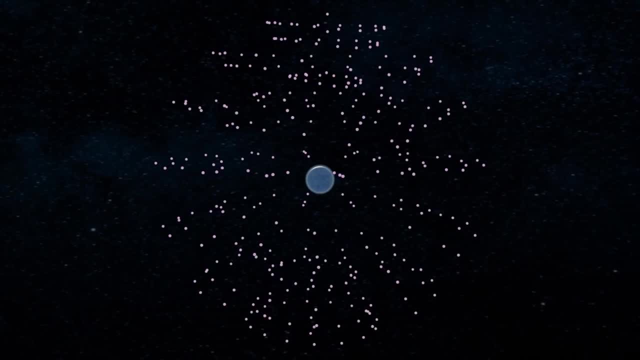 towards the central mass as time progresses, ie we have reproduced a classical gravitational field. So not only can we bring a three dimensional spacesurpose inductor to an answer line, também an object, but we can also draw a cross-d Gemini-Beneatr Roze to the focalwheel. 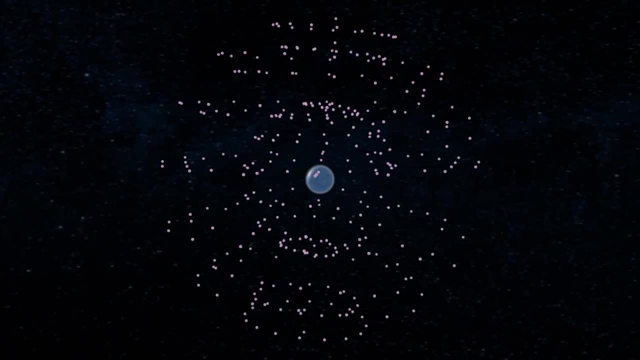 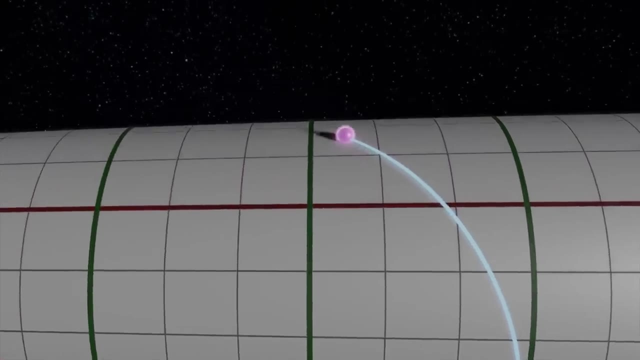 Actually we could sort of create something similar, but that same obligation would be safe for a gravitational field. So we can see how the geometry of spacetime helps create the illusion of gravity. But what happens if the curvature of our manifold becomes so great that there exists a limit? 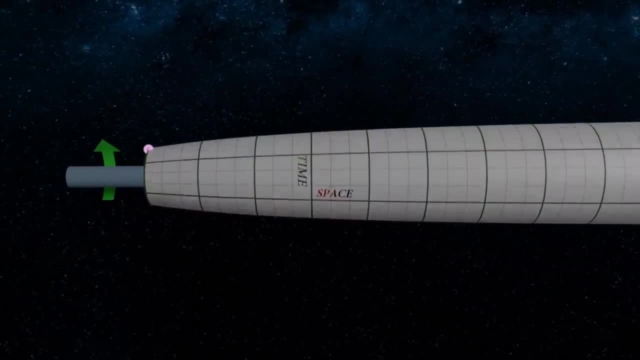 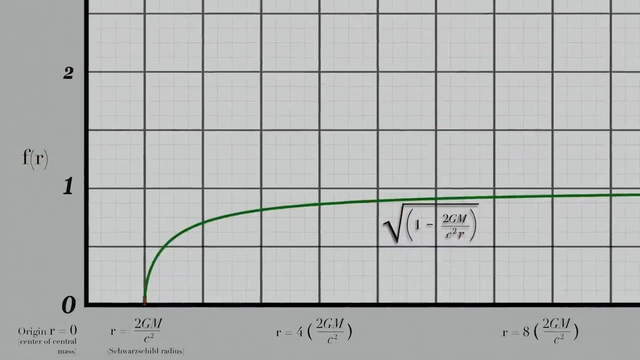 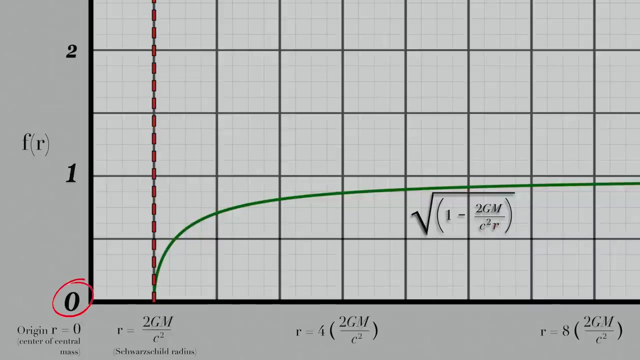 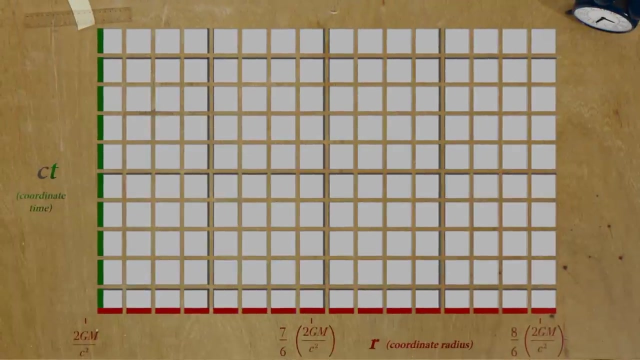 of no return. Well, returning to our Schwarzschild metric, we see that, for a certain value of the r coordinate, the temporal component of the metric goes to zero, while the spatial one blows up to infinity In terms of resizing our map, this means that pieces near this r coordinate value will become 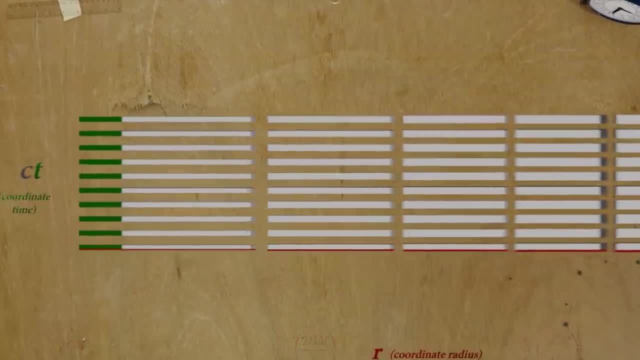 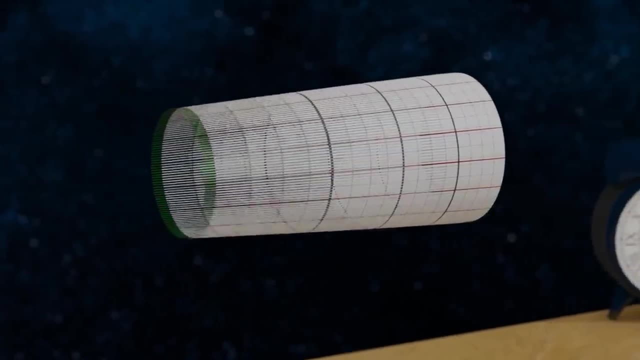 extremely thin and long When constructing the surface. then we can't be sure if it is a real or a real-world phenomenon, but we can easily assume that it is a real-world phenomenon again. these pieces will ultimately converge at a single point: sealing off the spacetime. 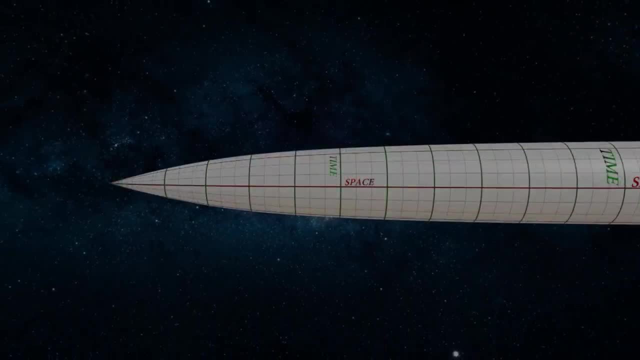 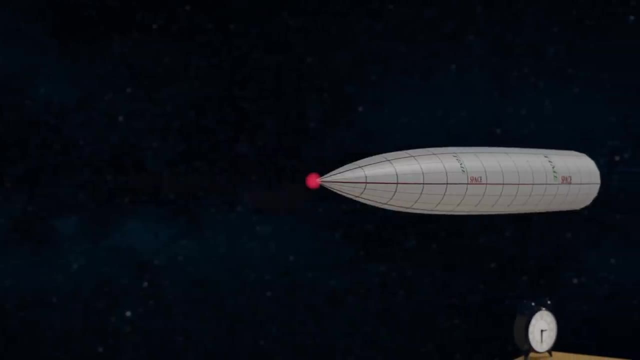 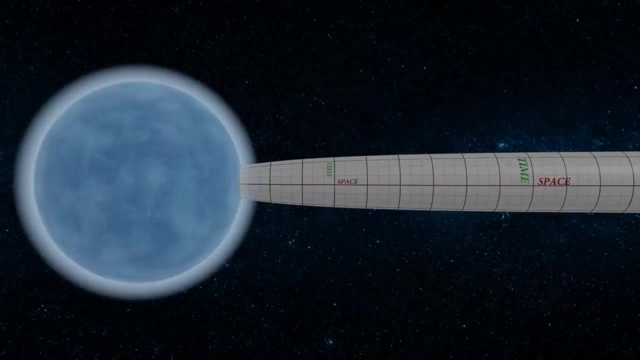 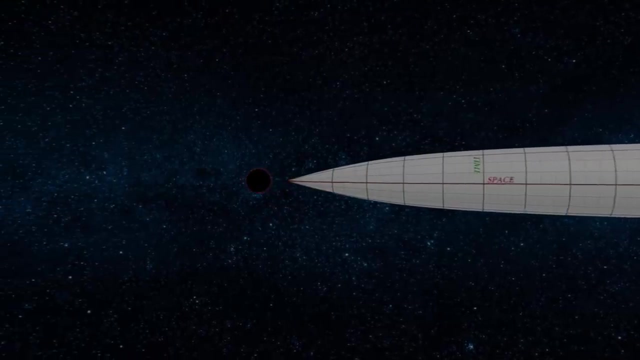 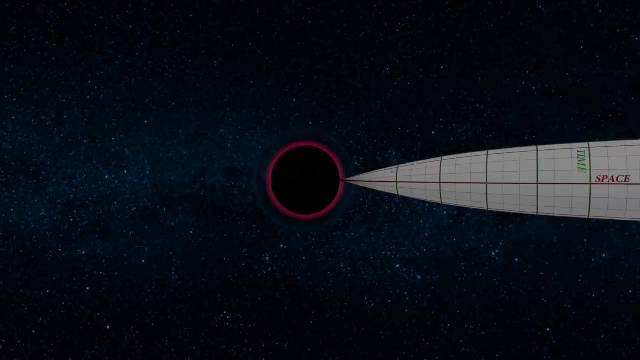 manifold there. This point is quite literally the point of no return: the object's event horizon. If this object is heavy and dense enough, the event horizon will lie exterior to its mass and it will be dubbed a black hole. Let's again look at the motion of two observers, but now near this manifold's event horizon. 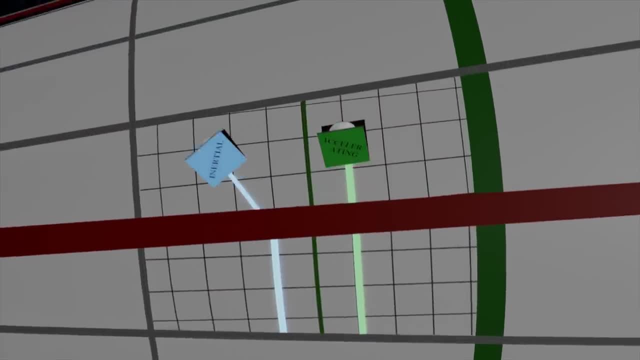 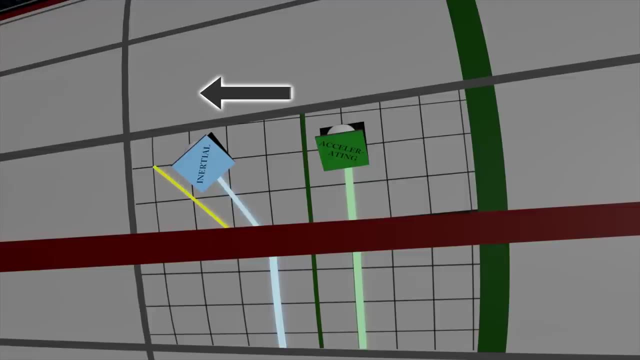 As they cross from one instant to the next. the worldline of the free-falling observer will be deflected by an amount almost equal to the worldline of light. In other words, the accelerated observable will be deflected by an amount almost equal. 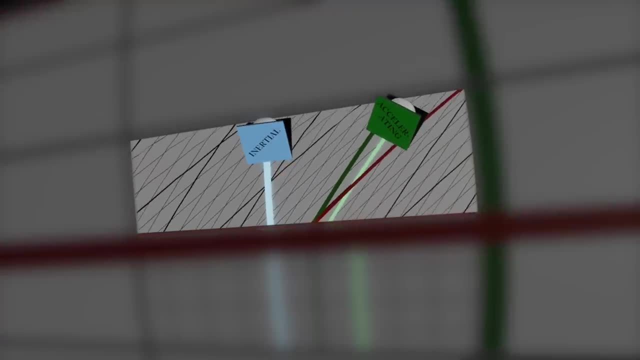 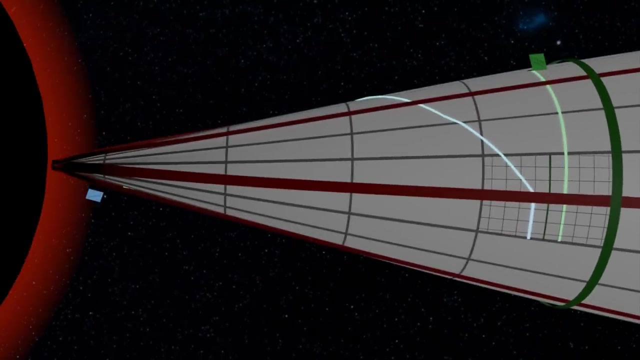 to the worldline of light. The observer's velocity has to increase by nearly the speed of light in order for them to remain at a stationary radial distance. Once the inertial observer falls past the event horizon, their speed is essentially now faster than the speed of light, at least relative to the observers outside the event.